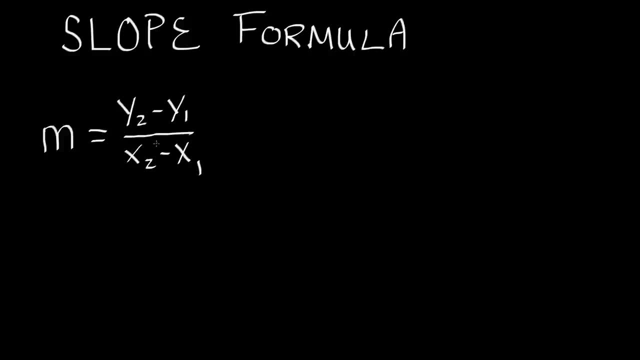 So what in the world is y2, y1, x2, x1? Where did those values come from? So, basically, y2 and y1 and x2 and x1, those are going to be components of the two points that we're going to use. 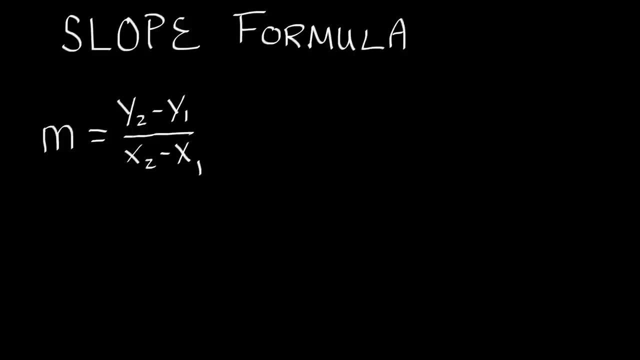 So basically, we're going to have one of our points and we're just going to call it P1 right now. So P1 stands for point 1. And for a point in the xy coordinate system, we basically need an x component and we need a y component. 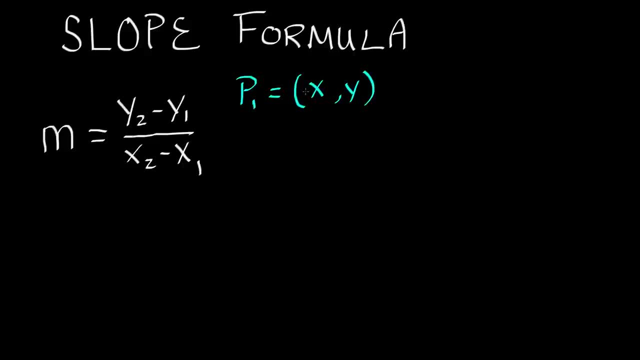 And since this is P1,, point 1, we're going to call our coordinates x1 and y1.. And so point 2, we're going to, We're going to refer to as P2, and we're going to go ahead and give it coordinates x2 and y2.. 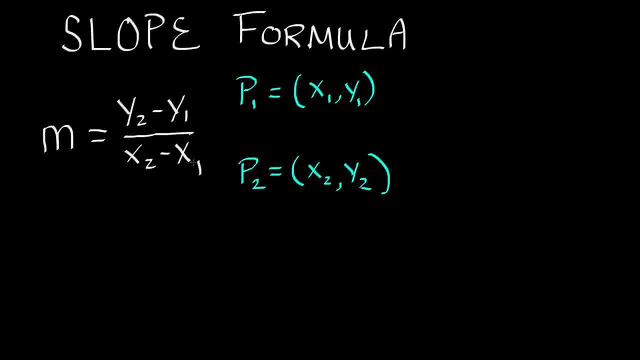 So this is where our y2,, y1,, x2, and x1 come from. They're basically coming from the points that we're going to be using, And these points are from the line that we're trying to find the slope of. 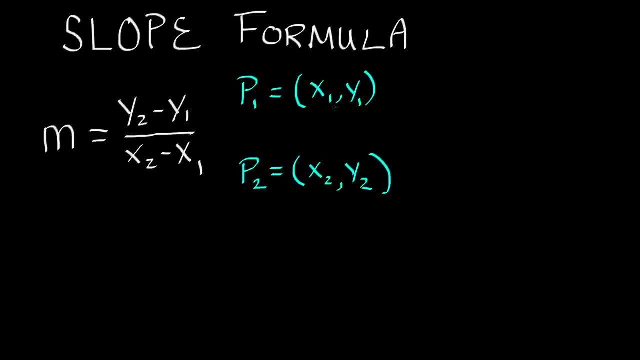 So let me just go ahead and just draw a coordinate system with a line on it, really quick. So now we've got this xy coordinate system And we've got this line as well, And then there's also these two points that are given to us, that are on the line. 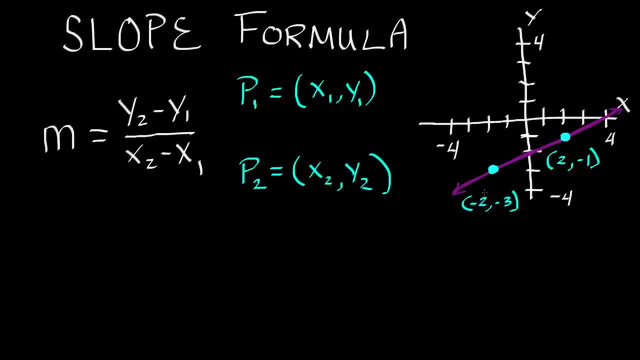 So now we basically just need to use this information from these two points to determine the slope of this line. So we need to figure out what y2,, y1,, x2, and x1 are. So we just need to pick one of these points to be point 1 and the other one to be point 2.. 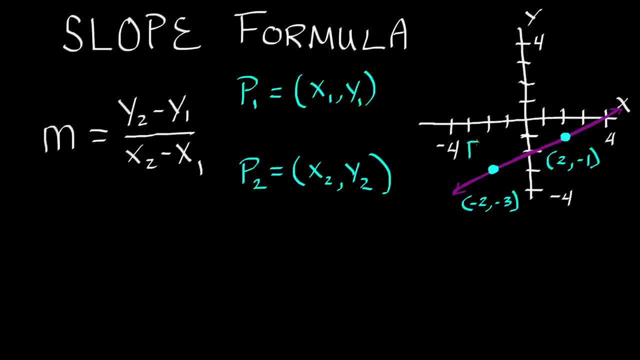 And it doesn't make a bit of difference Which one you pick to be which, So I'm just going to just choose this one to be point 1.. And then this one over here. I'll just call that one point 2.. 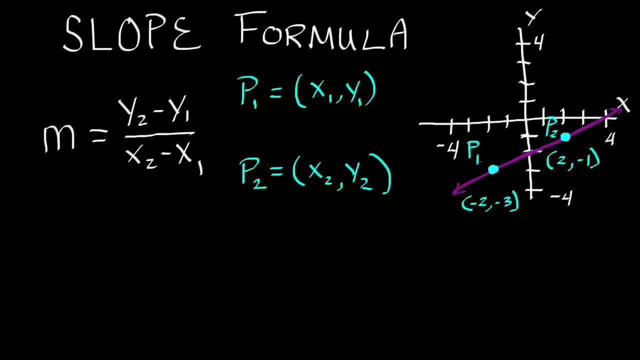 So, basically, you can pick either one to be point 2,, either one to be point 1.. You just need to make sure that you're consistent with the y2s and y1s and x2s and x1s in this formula. 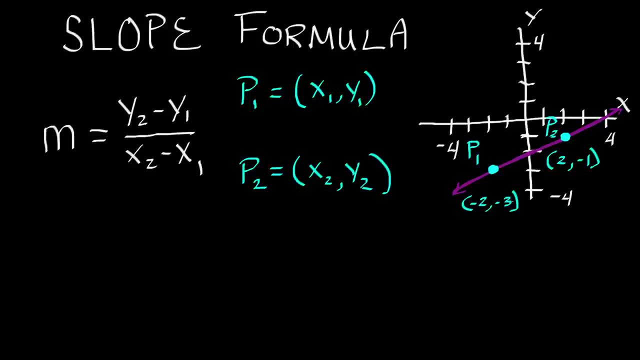 So basically, if this point negative 2, negative 3,, if that's p1, then we're going to have a point 2,, negative 3, and a point 2.. And then we're going to have a point 2,, negative 3, and a point 2.. 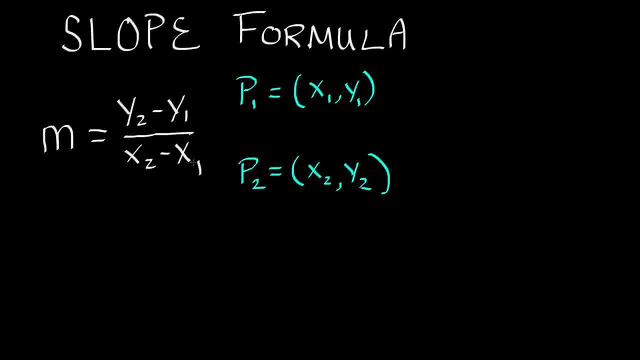 So this is where our y2,, y1,, x2, and x1 come from. They're basically coming from the points that we're going to be using, And these points are from the line that we're trying to find the slope of. 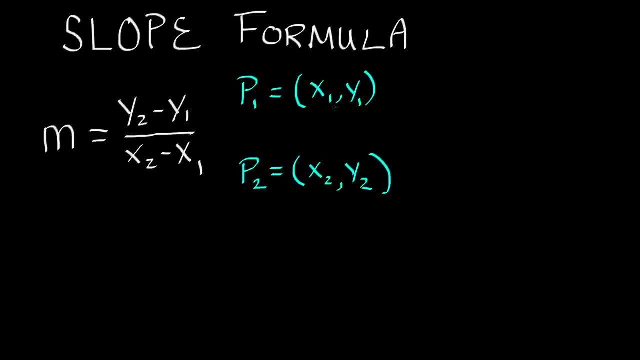 So let me just go ahead and just draw a coordinate system with a line on it, really quick. So now we've got this xy coordinate system And we've got this line as well, And then there's also these two points that are given to us, that are on the line. 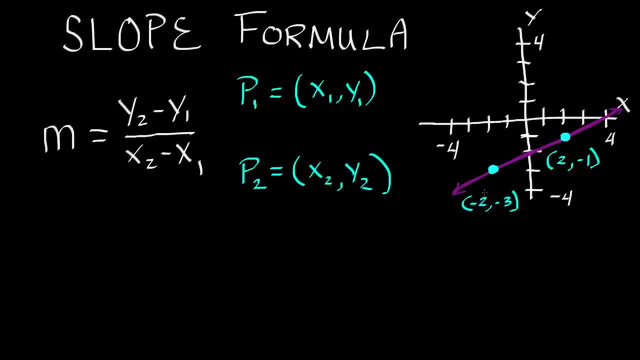 So now we basically just need to use this information from these two points to determine the slope of this line. So we need to figure out what y2,, y1,, x2, and x1 are. So we just need to pick one of these points to be point 1 and the other one to be point 2.. 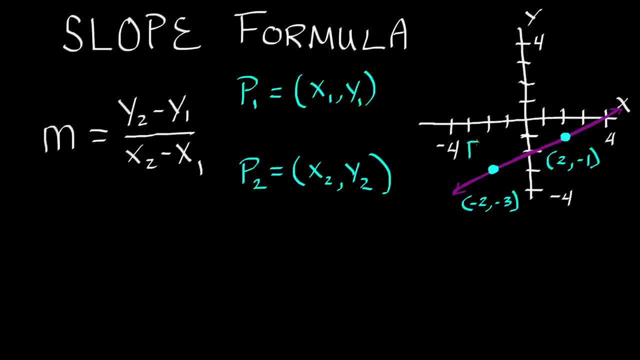 And it doesn't make a bit of difference Which one you pick to be which, So I'm just going to just choose this one to be point 1.. And then this one over here. I'll just call that one point 2.. 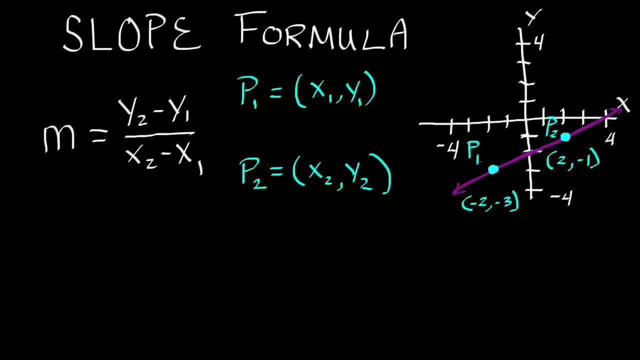 So, basically, you can pick either one to be point 2,, either one to be point 1.. You just need to make sure that you're consistent with the y2s and y1s and x2s and x1s in this formula. 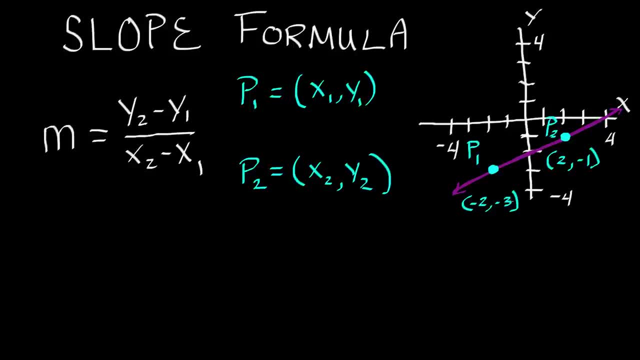 So basically, if this point negative 2,, negative 3, if that's p1, then we're just going to go ahead and just put that up here for p1. We're just going to put negative 2,, negative 3.. 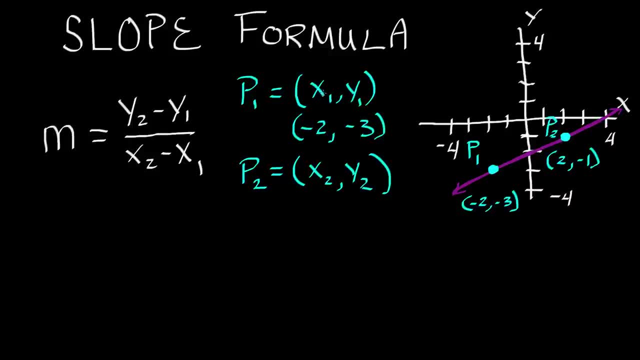 So now do you see that x1 has a value of negative 2?? y1 has a value of negative 3.. So p2 is the other point. It's 2, negative 1.. So we'll just go ahead and put 2, negative 1.. 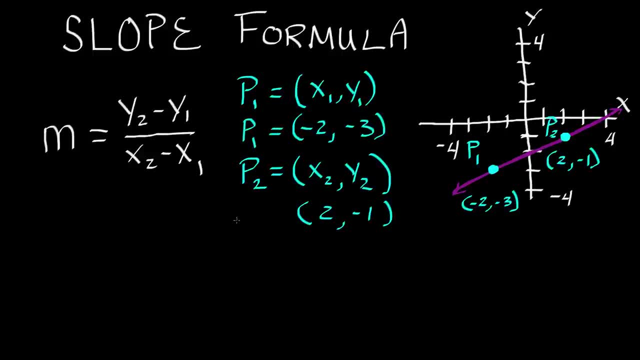 And then I'll just go ahead and put p1 up here, just for clarity, And p2. p2 down here. So basically, x2 is equal to 2 now And y2 is equal to negative 1.. So now what we need to do is we just need to translate the y2, y1, x2, and x1. 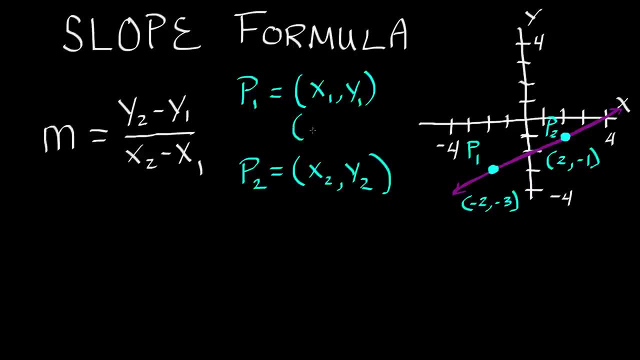 We're just going to go ahead and just put that up here for p1.. We're just going to put negative 2, negative 3.. So now do you see that x1 has a value of negative 2? y1 has a value of negative 3.. 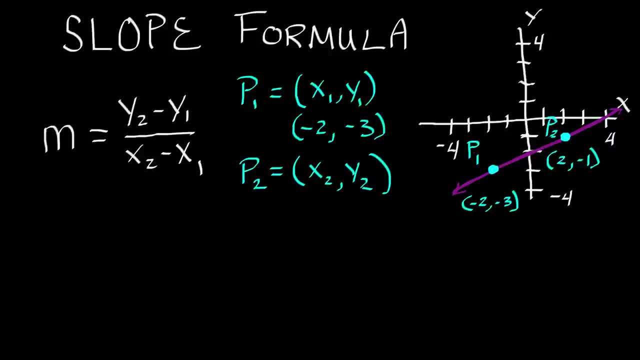 So p2 is the other point. It's 2, negative 1.. So we'll just go ahead and put 2, negative 1.. And then I'll just go ahead and put p1 up here, just for clarity, And p2 down here. 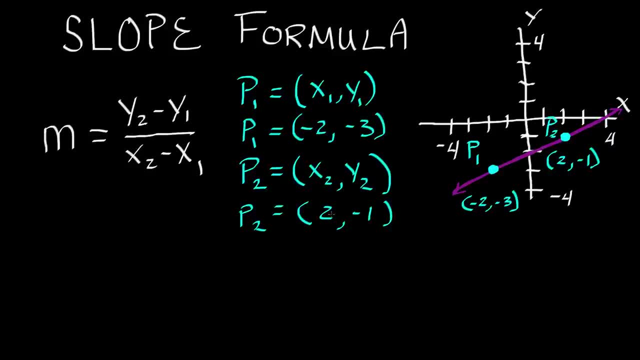 So basically, x2 is equal to 2 now, And y2 is equal to negative 1.. So now what we need to do is we just need to translate the y2,, y1, x2, and x1 to the numbers that we have represented here by those components. 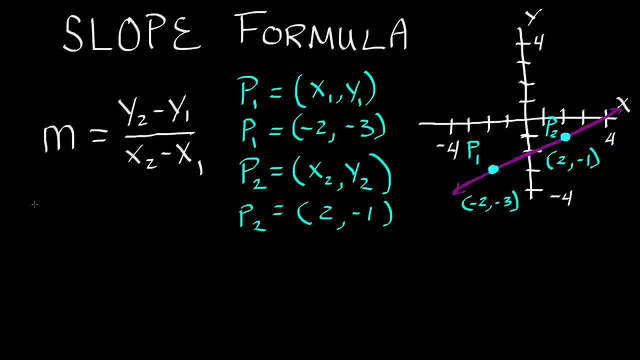 and plug it into the slope formula. So now we're basically looking at our slope is equal to now y2, y2 is the right-hand side of the p2 point. So y2 corresponds to that negative 1 right here. So we put negative 1 for y2.. 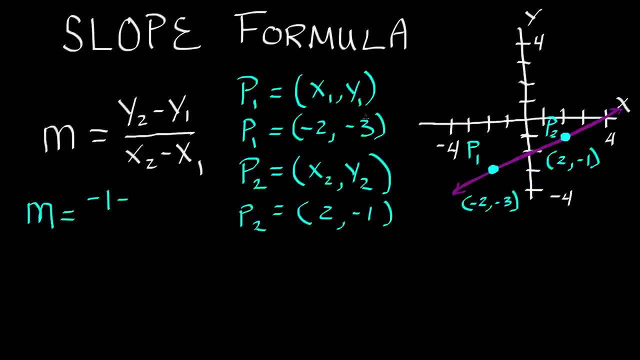 And then we're subtracting y1.. So y1, we go up here to point 1.. And the y1 component corresponds to the negative 3 in p1.. So we're subtracting a negative 3.. And then we're dividing that by x2 minus x1.. 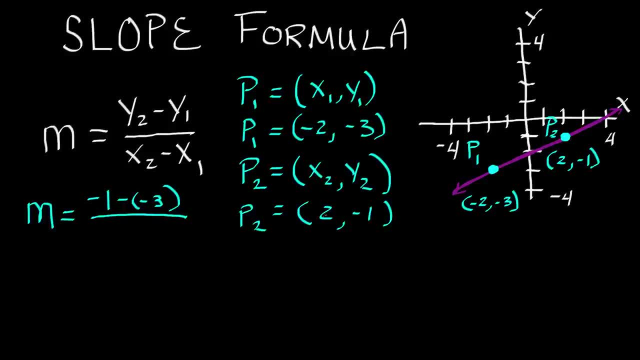 So x2 comes from point 2.. And x2 represents this 2 right here. So we'll just put 2 for x2.. And then we subtract x1.. So subtracting x1, x1 is up here with point 1.. 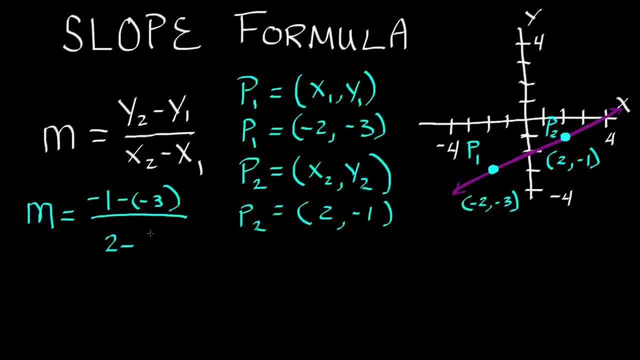 And x1 corresponds to the negative 2.. So we're subtracting a negative 2.. So now we basically have negative 1 minus a negative 3.. And so minus a negative is the same thing as plus. So we're just going to rewrite this as m is equal to minus 1 plus 3.. 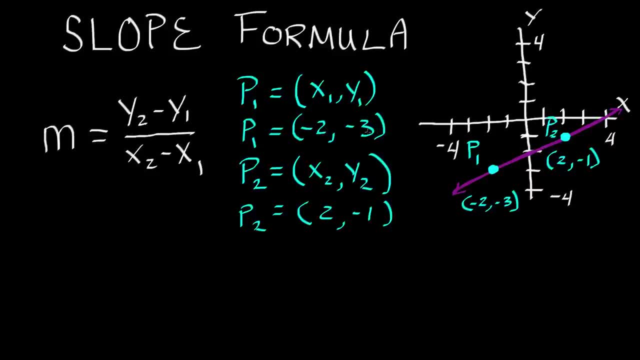 to the numbers that we have represented here by those components and plug it into the slope formula. So now we're basically looking at our slope. So our slope is equal to now y2,. y2 is the right-hand side of the p2 point. 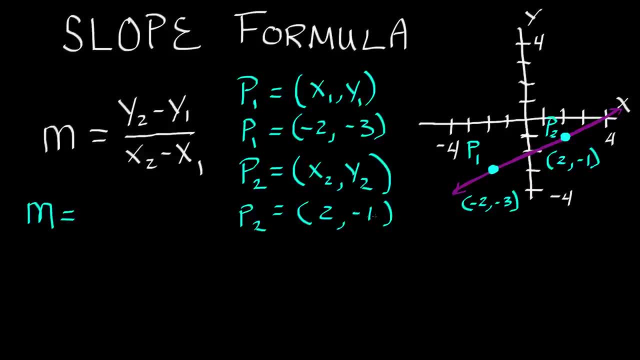 So y2 corresponds to that negative 1 right here. So we put negative 1 for y2.. And then we're subtracting y1.. So y1, we go up here to point 1.. And the y1 component corresponds to the negative 3 in p1. 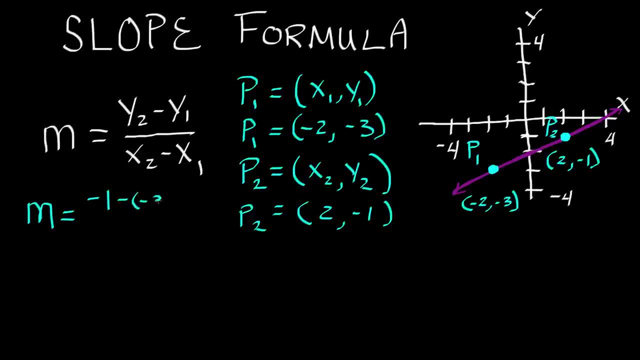 So we're subtracting a negative 3. And then we're dividing that by x2 minus x1.. So x2 comes from point 2. And x2 represents this 2 right here. So we'll just put 2 for x2.. 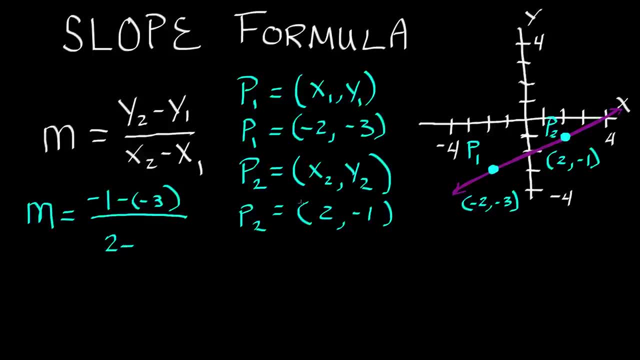 And then we subtract x1.. So subtracting x1, x1 is up here with point 1.. And x1 corresponds to the negative 2. So we're subtracting a negative 2.. So now we basically have our slope. 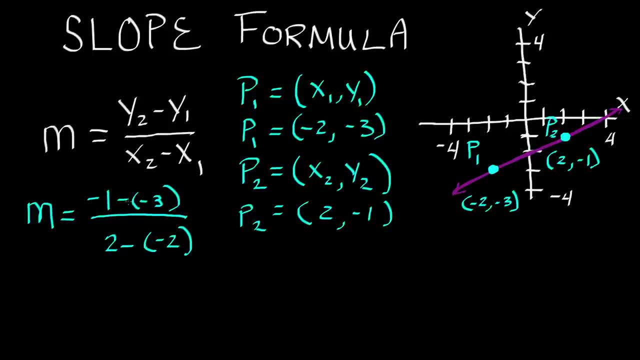 So now we basically have negative 1 minus a negative 3.. And so minus a negative is the same thing as plus. So we're just going to rewrite this as m is equal to minus 1 plus 3.. And then on the bottom, we have the same situation: 2 minus a negative 2.. 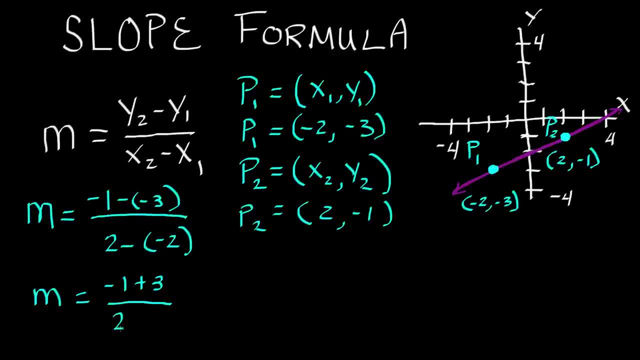 Well, minus a negative is a plus once again. So this ends up becoming 2 plus 2 on the bottom. And then we have negative 1. And we're adding 3 to that, But that becomes a positive 2. And on the bottom we have 2 plus 2, which is equal to 4.. 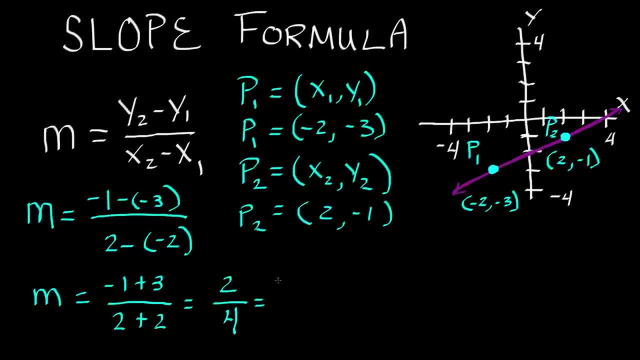 So 2 over 4 now can be reduced. So 2 is the same thing as 2 times 1.. And 4 is the same thing as 2 times 2.. So now our 2 and 2 cancel right here, leaving us. 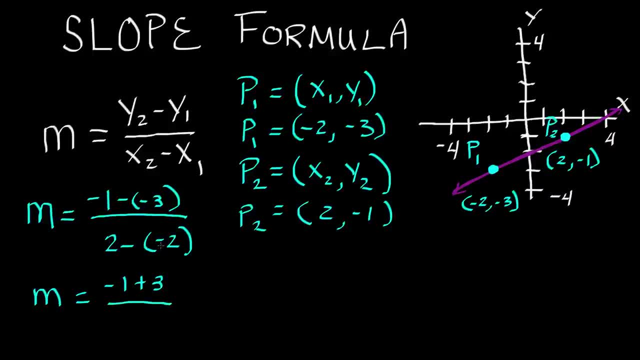 And then on the bottom we have the same situation: 2 minus a negative 2.. Well, minus a negative is a plus once again. So this ends up becoming 2 plus 2 on the bottom, And then we have negative 1..